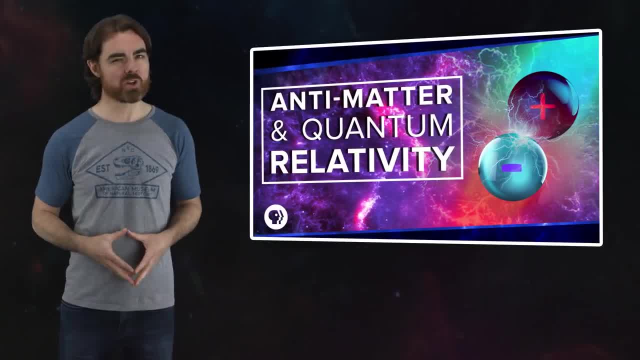 We covered the Dirac equation last time, and you really should watch that episode first if you haven't already. 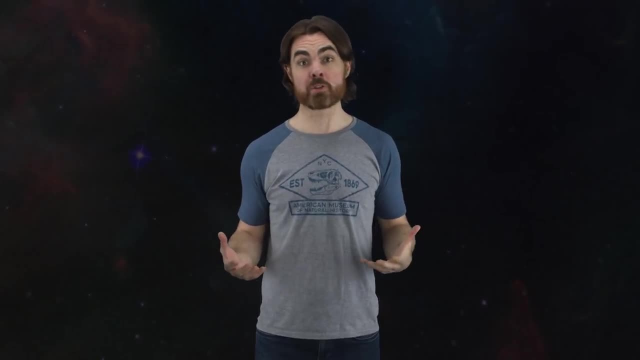 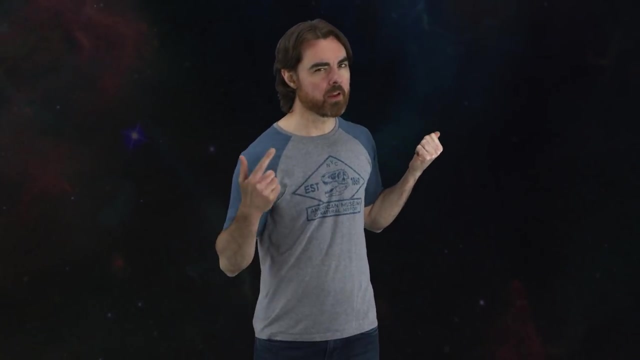 Now, before we start thinking about vibrating quantum fields, or even fields at all, let's talk about vibrations. Anyone who's ever strummed or shredded knows that a stretched string vibrates with a certain frequency when plucked. 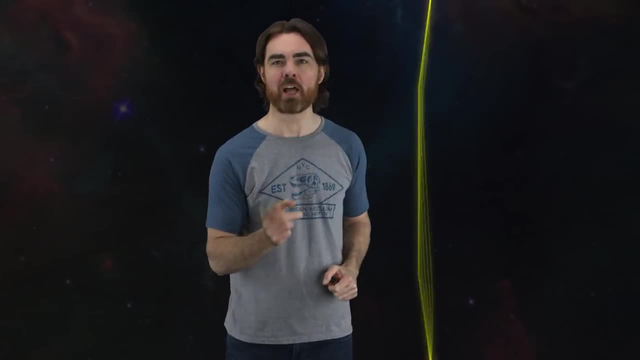 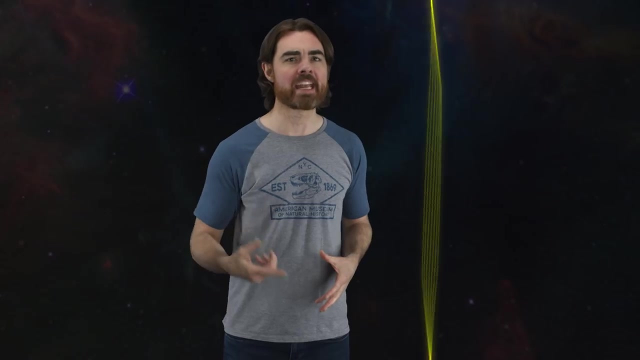 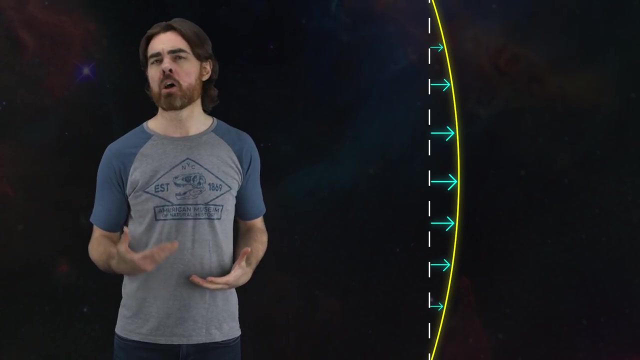 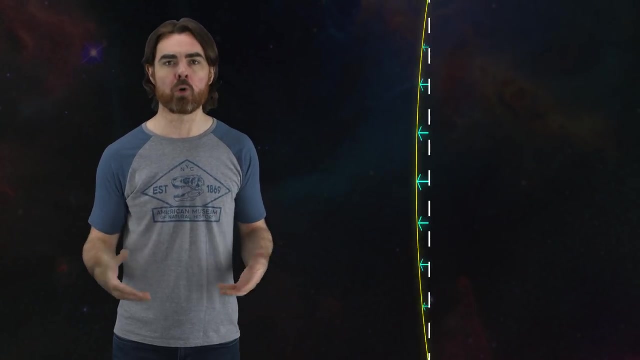 It also vibrates with an amplitude that depends on how hard you pluck it. A larger amplitude and or larger frequency means the vibration carries more energy. At any point in time, every point on a vibrating string is displaced by some distance from its relaxed or equilibrium position. And that displacement changes over time as the string oscillates back and forth. 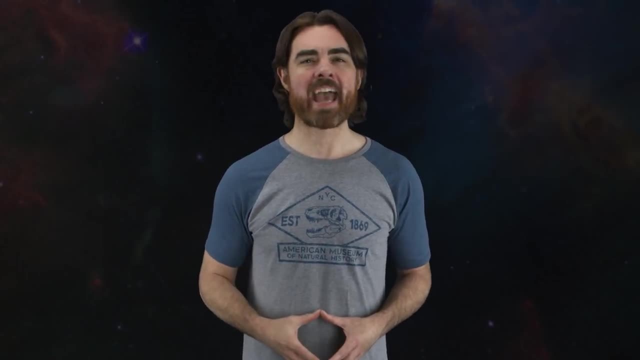 Guitar strings are one-dimensional, but we can expand the analogy to any number of dimensions. 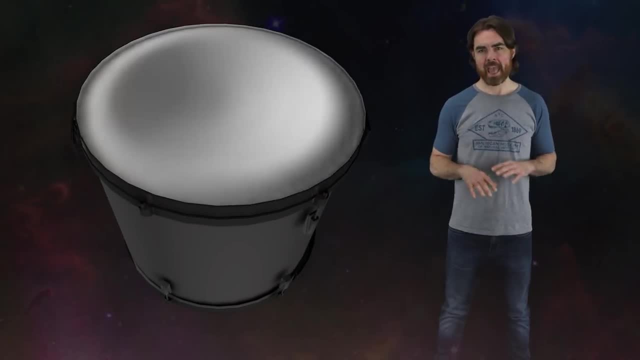 In 2D, we have a membrane, like a drum skin. Everywhere on the surface of a vibrating drum skin, there's a displacement from the flat equilibrium state in the up-down direction. The 3D analogy is harder to imagine. 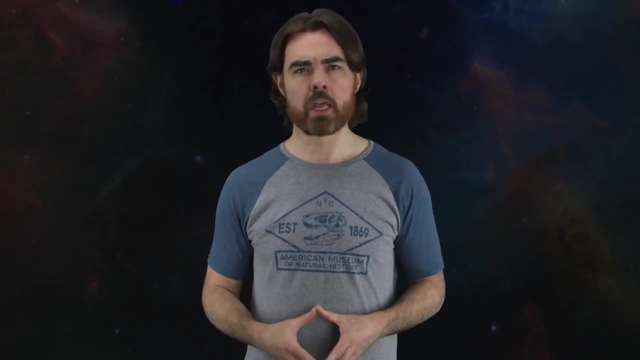 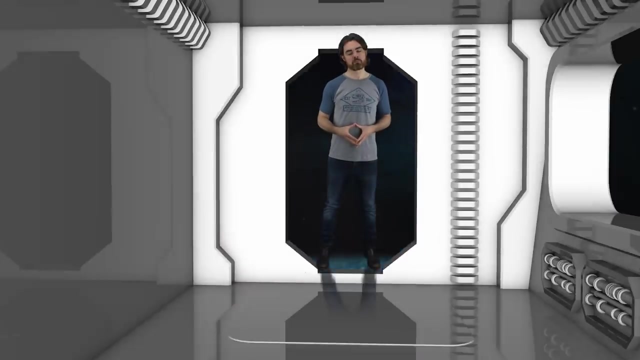 Every point in space has some displacement in some imaginary extra direction, analogous to, but not the same as, a fourth dimension. 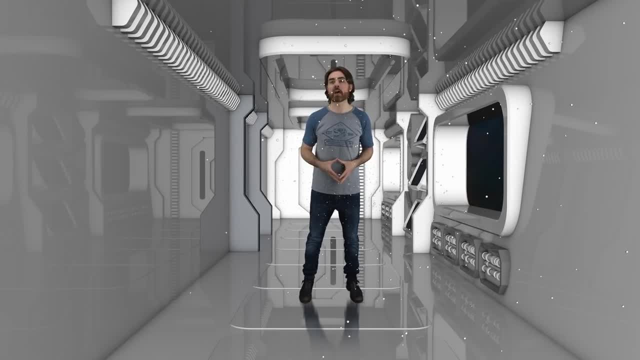 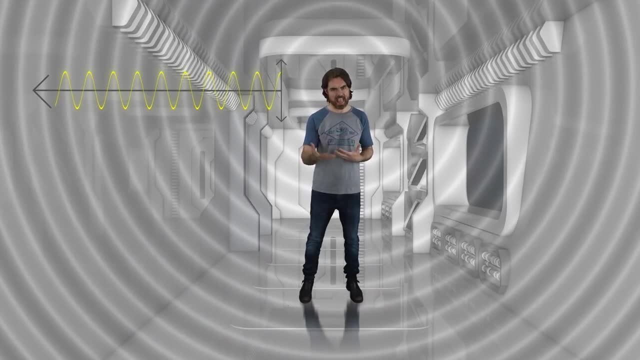 For example, in a 3D room full of air, sound waves are oscillations in air density. That air density has an equilibrium value, which is just the average density. But at every point in the room, a sound wave can cause air density to oscillate to higher and lower values. 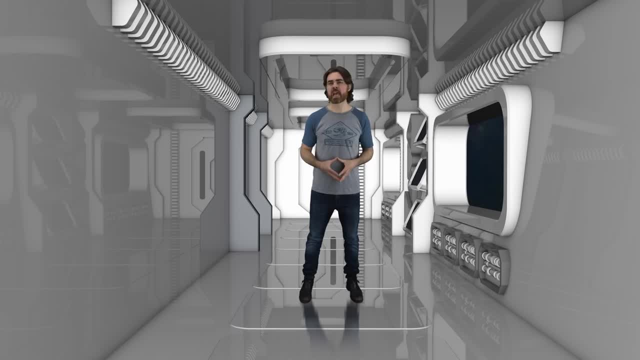 We describe air density as a field, because it has some value everywhere in the space of the room. 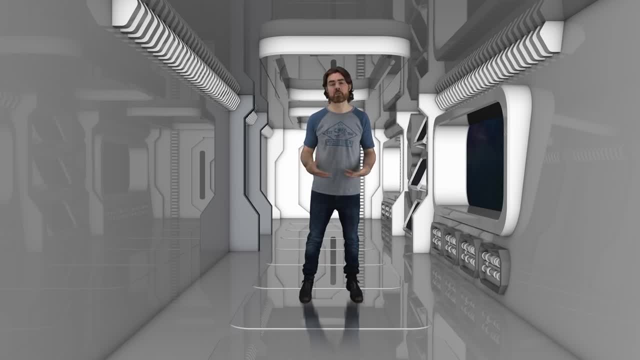 And that's all a field is, some property that has some value throughout a space. 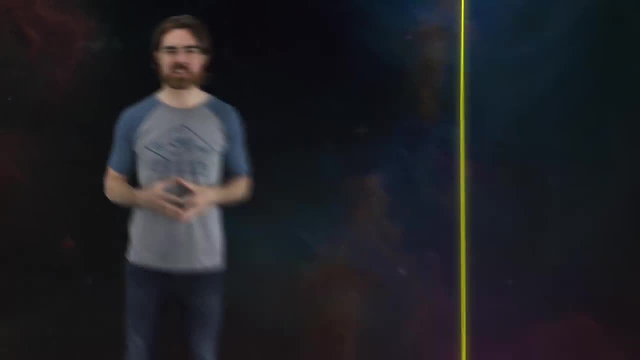 OK, let's go quantum. And let's go back to the string. 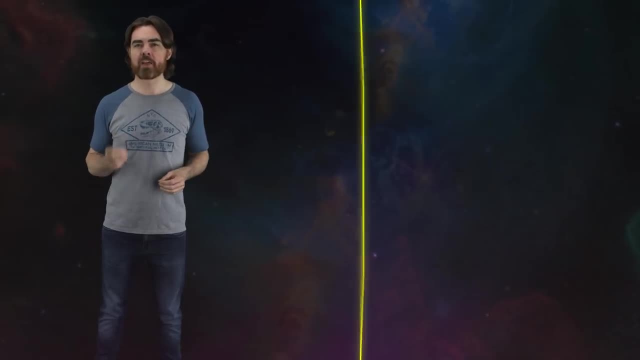 If this were a quantum mechanical guitar string, then there'd be a minimum amplitude for the vibration that depended on its frequency. No vibrations with amplitudes smaller than that minimum could exist. 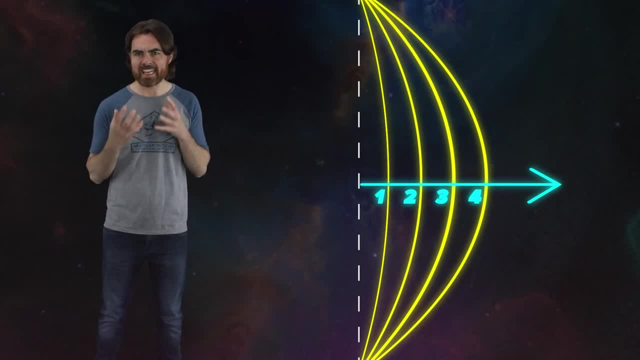 And every larger vibration would have to be a whole number, an integer multiple of the smallest amplitude. 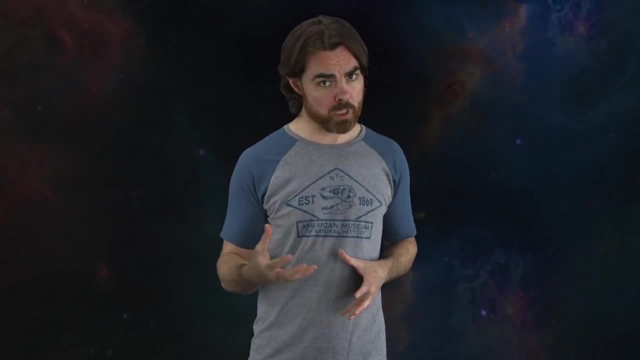 This is exactly how light behaves, as was first realized by Max Planck and proved by Einstein. 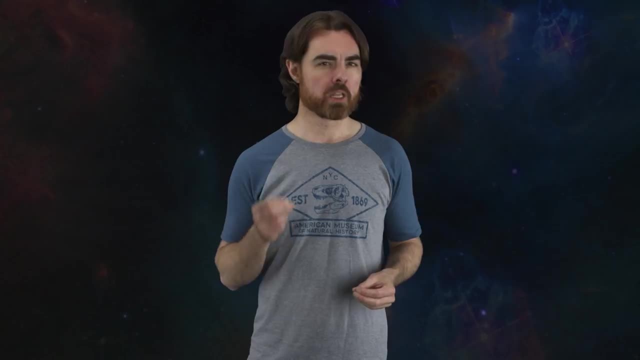 Light is a wave in the electromagnetic field. The electromagnetic field is similar to the density field in a room full of air. It has a value, a field strength, everywhere in the universe. OK. 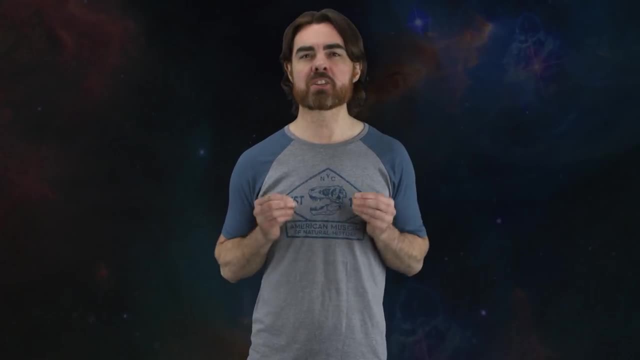 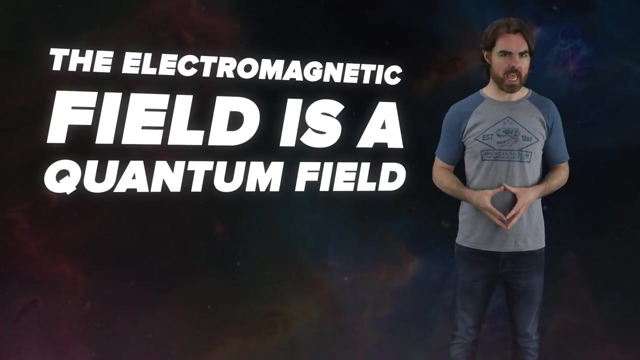 That value is usually 0. But just like the string or the air density field, it could oscillate. The electromagnetic field is a quantum field. And so these oscillations have a minimum amplitude. The smallest possible oscillation above 0 is an indivisible little packet of energy that we call a photon. Quantum physics may have started with Planck's discovery 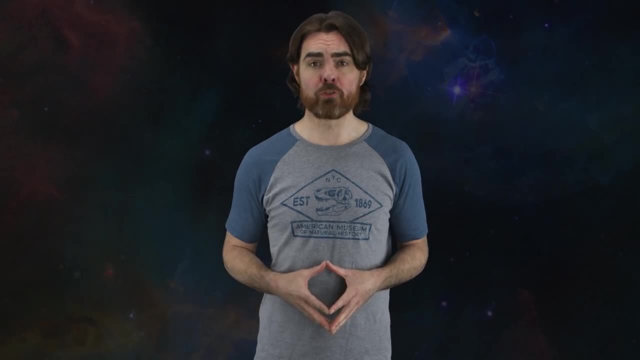 of the quantum nature of light. However, the first full formulation of quantum mechanics was Schrodinger's equation. 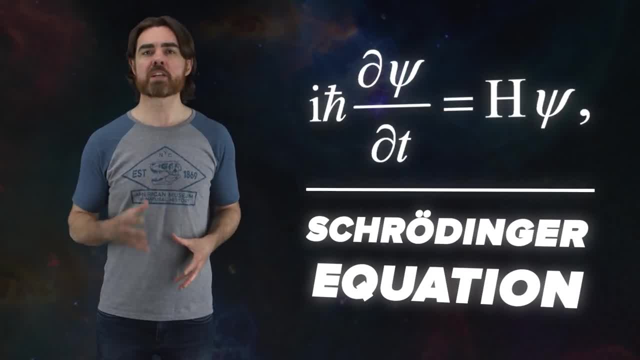 And it couldn't account for light at all. We touched on the reason for that in last week's episode. 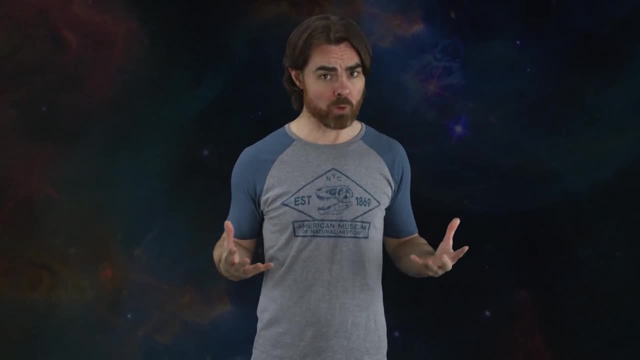 Basically, the Schrodinger equation is incompatible with Einstein's relativity. It can't describe things moving anywhere near the speed of light. 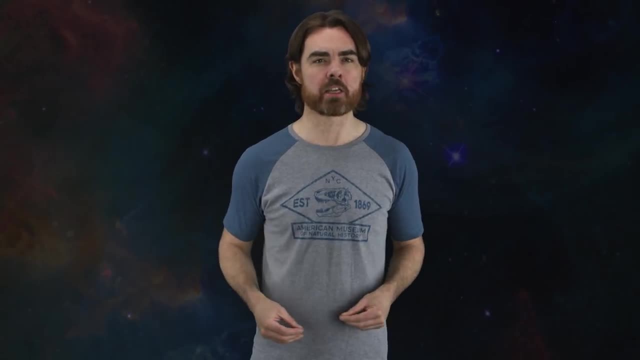 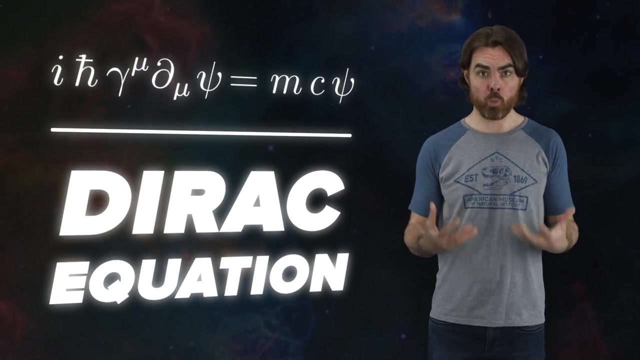 And it implicitly assumes that forces act instantaneously. We also saw how Paul Dirac managed to find an equation describing the behavior of the electron that worked. 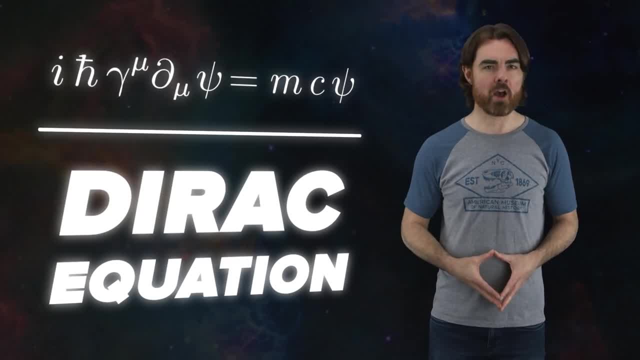 With relativity, the Dirac equation. However, understanding the behavior of light and its interaction with matter required a different approach. 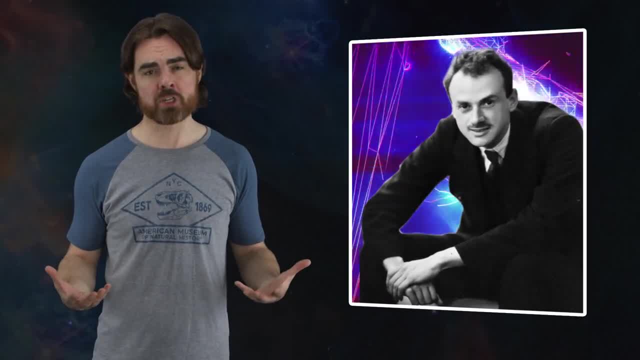 It also required Paul Dirac. Again, that guy was a genius. 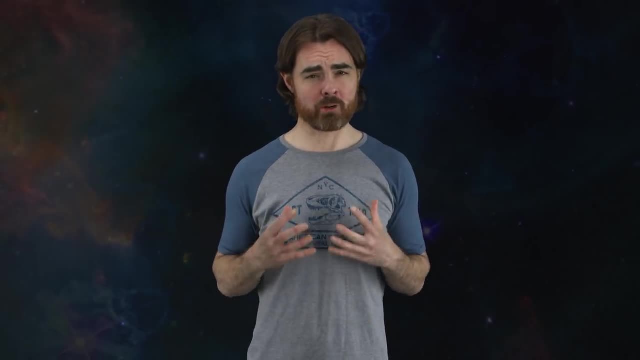 Let me first mention another problem with the Schrodinger equation. It's terrible for many particle systems. It follows the changing position and momentum and generally the physical quantum state of every individual particle. 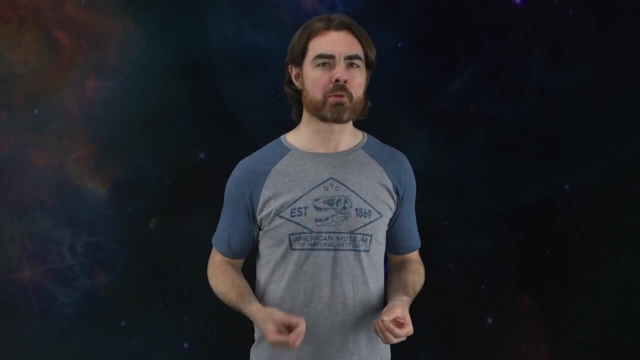 But that's extremely inefficient. See, two of the same type of elementary particle are indistinguishable from each other. 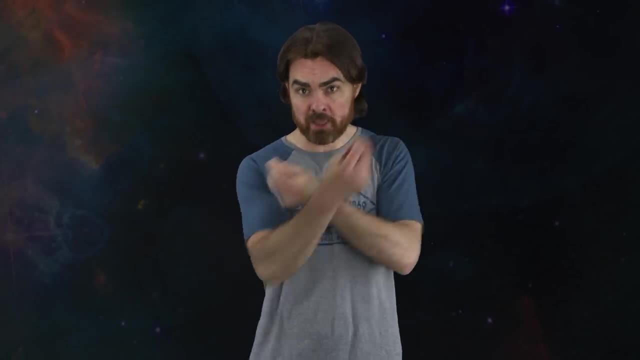 If you take a pair of electrons or photons in two quantum states and make them swap places, then nothing changes. 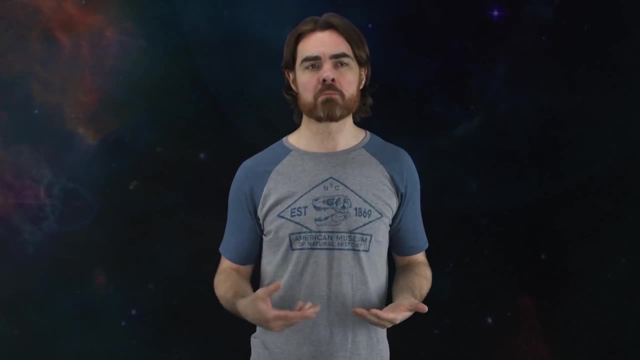 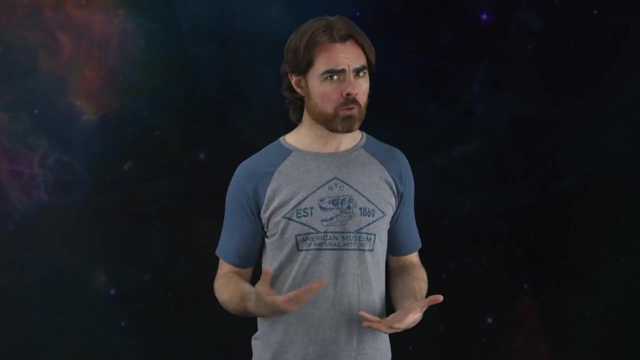 Following the quantum state of every individual particle is like trying to do your finances by tagging and tracking the movement of each individual dollar. No one cares which dollar is which. We only care how many dollars end up in whose bank account. 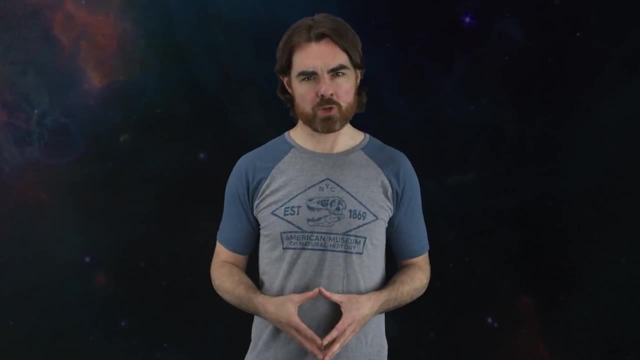 But bean counting this way is not just inefficient in quantum mechanics. It gives the wrong answers. 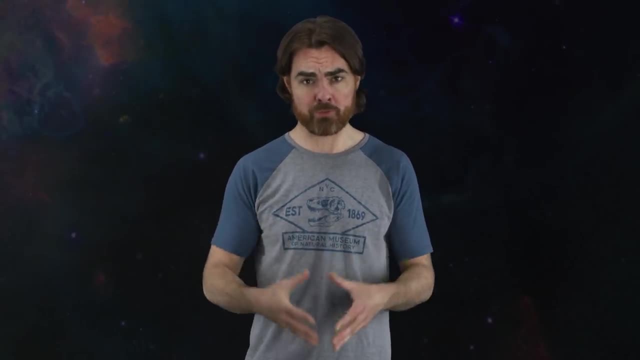 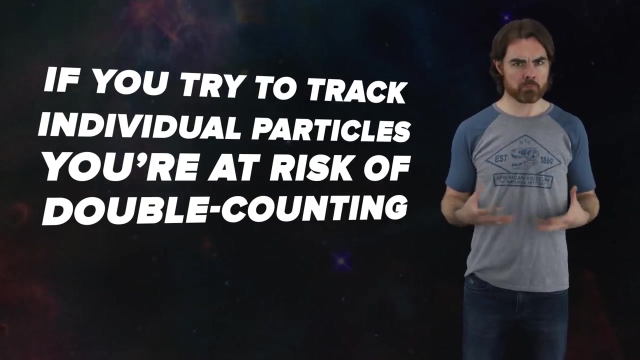 A given quantum event or interaction can happen in multiple different ways. And the probability of the interaction depends on correctly counting those different possible ways. If you try to track individual particles, you're at risk of double counting. You end up with multiple arrangements of particles that are actually the same arrangement due to the particles being identical to each other. That means you get the wrong probabilities. Paul Dirac's solution was to not try to track the changing states of individual photons. Instead of quantizing particles' physical properties like position and momentum, as did Schrodinger, Dirac quantized the electromagnetic field itself. He imagined each point in space as being an oscillator, technically. A simple harmonic oscillator, just like an oscillating spring. 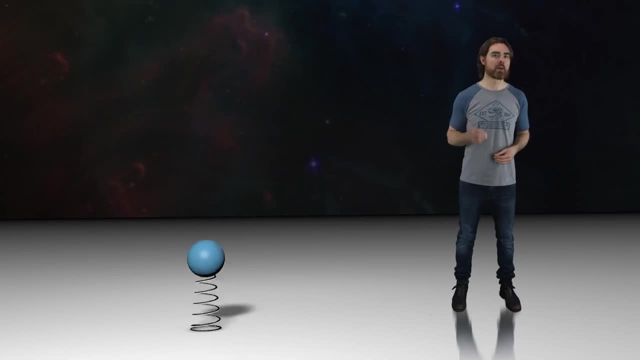 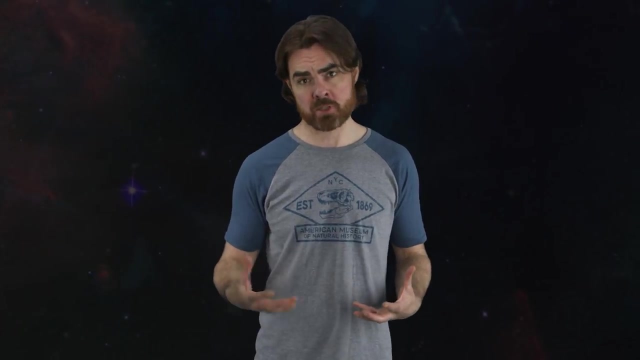 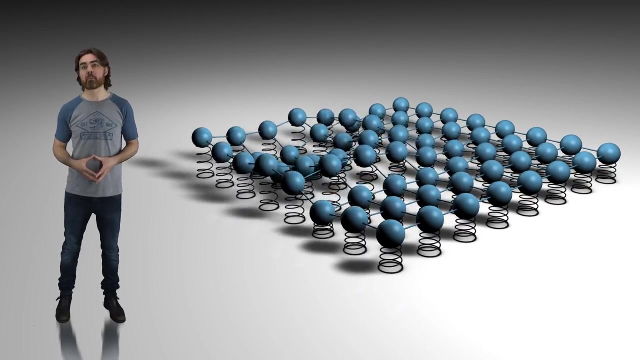 The oscillation at each point can be complicated, but it has to be built up from a number of minimum amplitude quantum oscillations, which is to say, photons. So Dirac described a space of quantum states, including position and momentum slash frequency, like an infinite array of springs. His mathematics then kept track of the number of particles or quantum oscillations in each of these states. 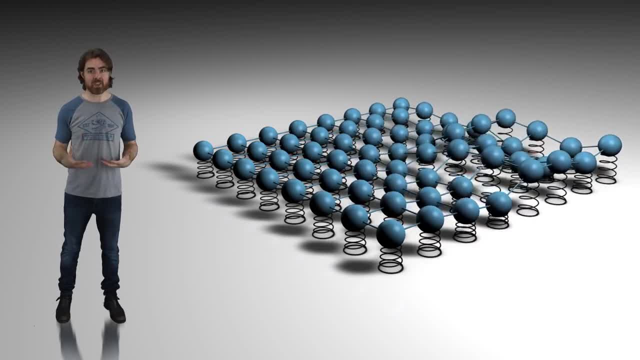 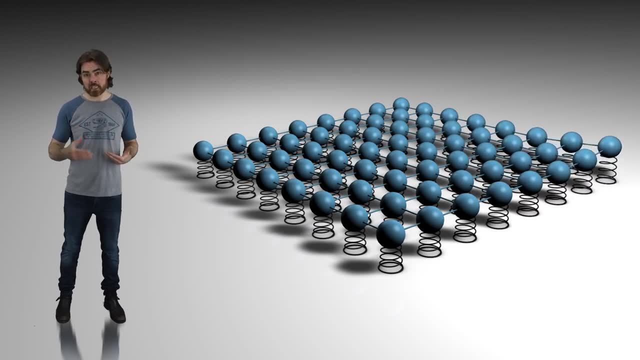 This automatically avoids double counting, because the math doesn't even try to keep track of the movement of individual photons, only the shifting number in each quantum state. 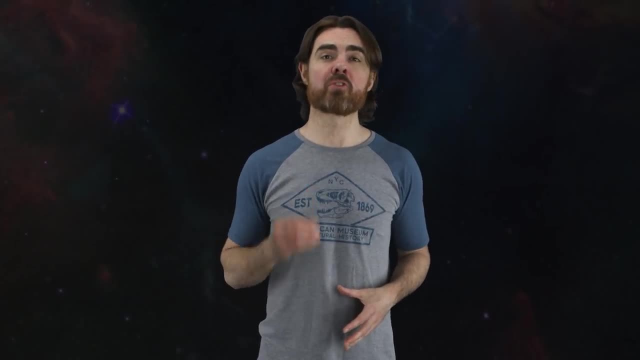 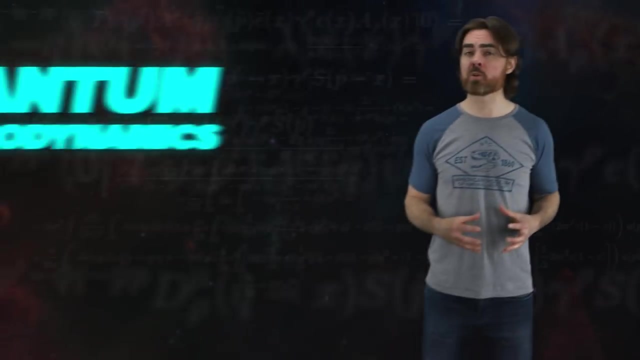 Dirac wasn't the first to come up with this idea, but he was the first to successfully apply it to describing electromagnetic interactions. He named the resulting theory quantum electrodynamics. dynamics. 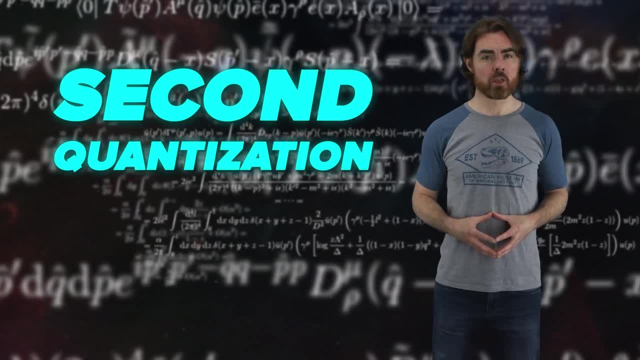 He also coined the name second quantization for the process of counting the changing number of quantum oscillations or particles per state. 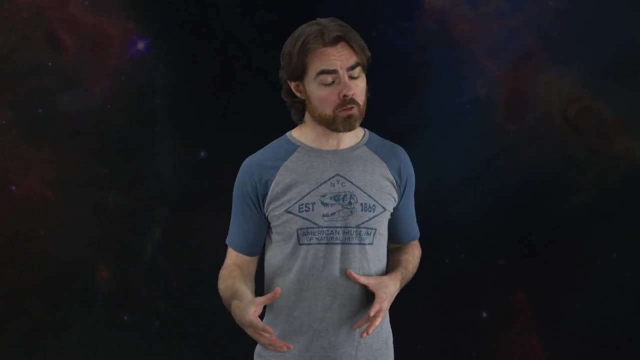 Schrodinger's approach of tracking the change in quantum state of each particle became the first quantization. 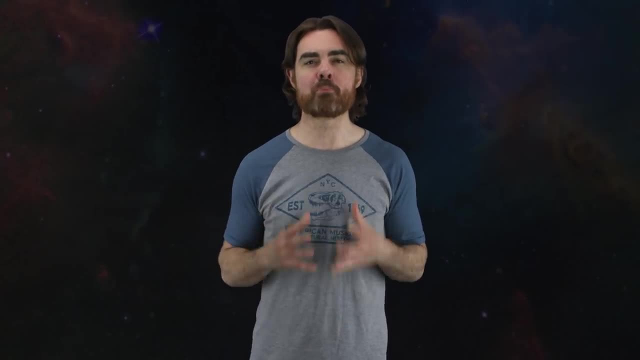 There's another reason this second quantization is better at describing the interactions of light and matter. 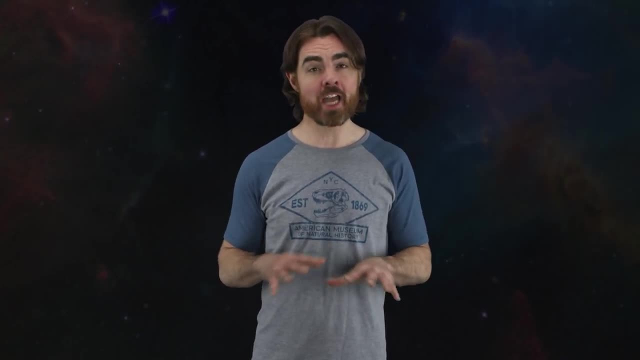 See, Schrodinger's approach has no idea how to destroy a particle. All it can do is move particles around 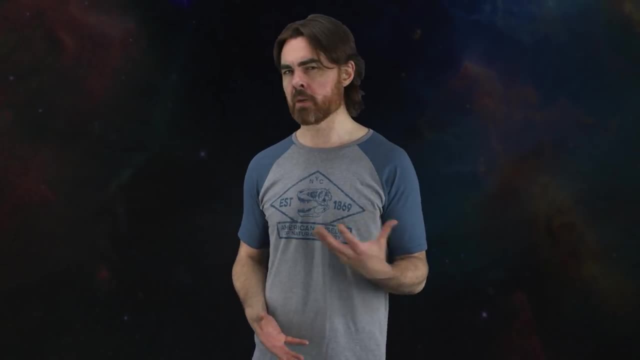 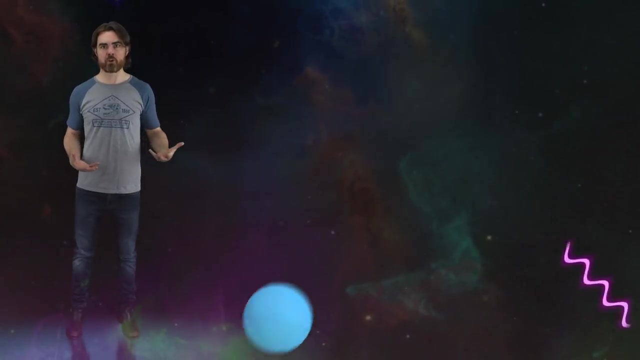 via their evolving wave functions. Yet in particle interactions, particles are created and destroyed all the time. An electron can absorb or emit a photon. An electron and a positron can annihilate each other and create two photons. And that can even happen the other way around. 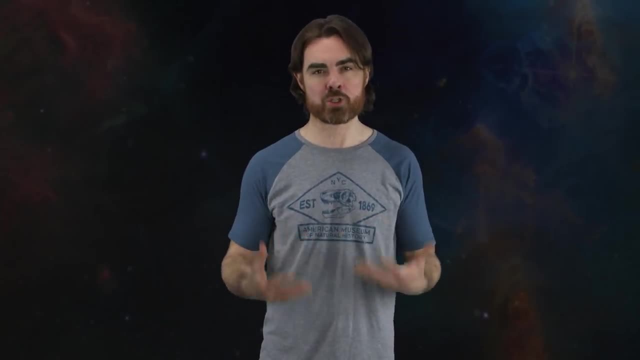 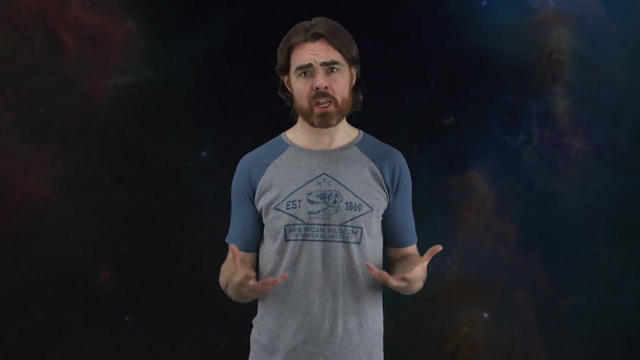 But the second quantization is all about creating and destroying particles. This new capability became essential for the description of subatomic processes. The resulting quantum electrodynamics describes the interactions of matter and radiation with stunning success. 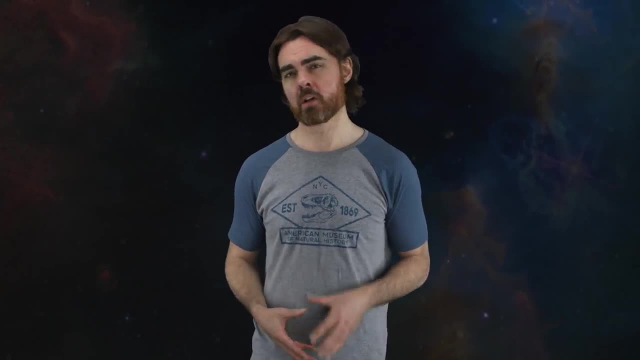 It is one of the most carefully tested theories in all of physics. 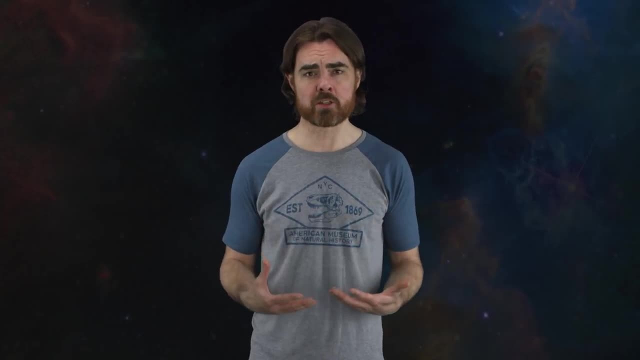 For example, it eventually allowed scientists to predict with incredible precision the tiny difference in atomic electron energy levels 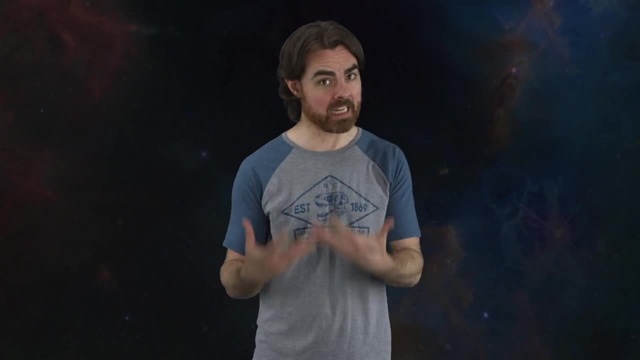 due to electron spins, spins interacting with magnetic fields. 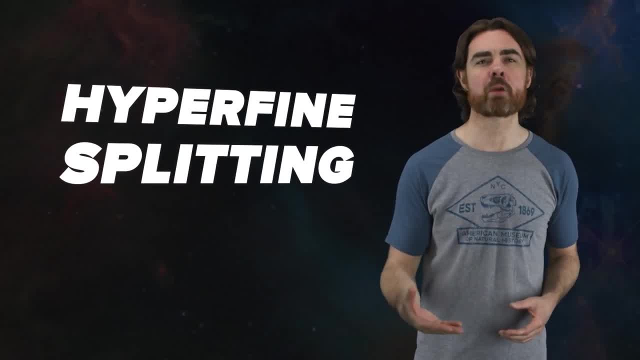 This is the first time that a particle is built in the so-called hyperfine splitting, or spins interacting with vacuum energy fluctuations in the Lamb shift. 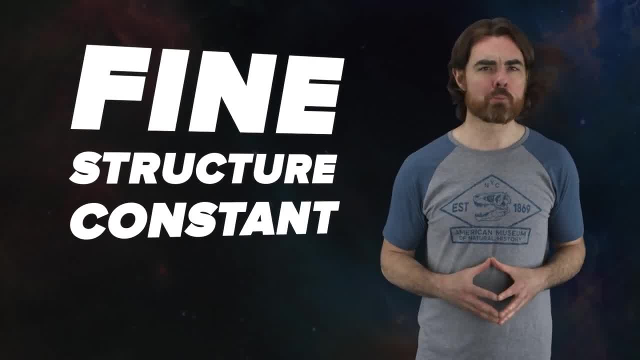 It predicts the relative value of the fine structure constant 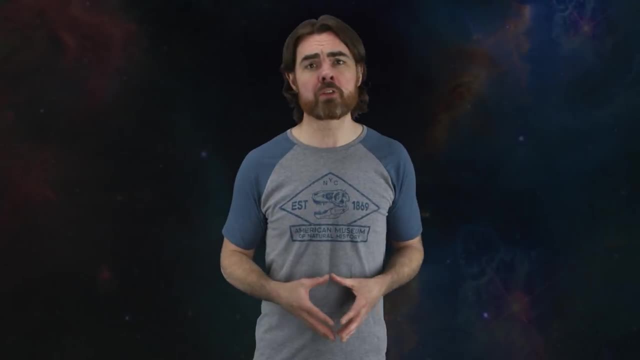 to a precision of one part in a billion. 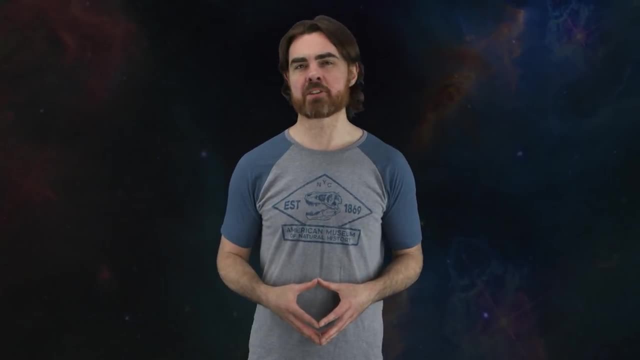 No other theory in physics has done so well. 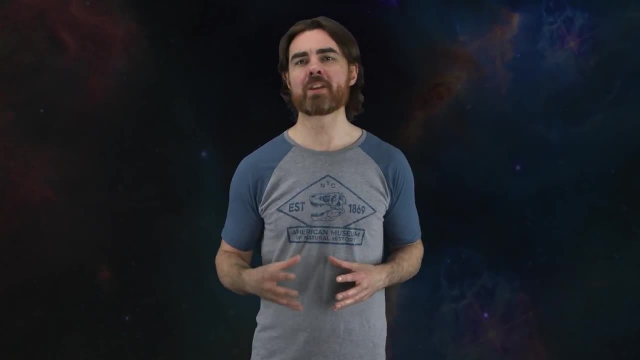 Spurred by its success in describing electromagnetism, physicists soon extended the second quantization approach 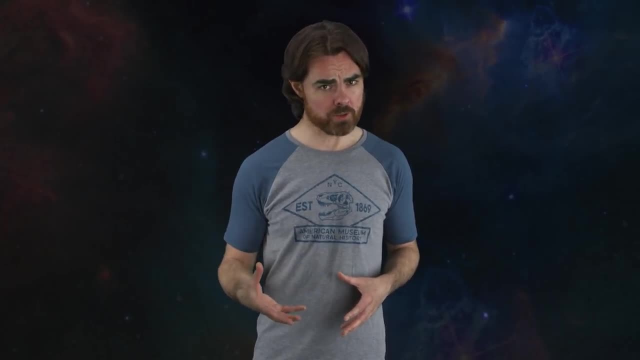 to other elementary particles. This is the first time that a particle is built in the so-called hyperfine splitting. 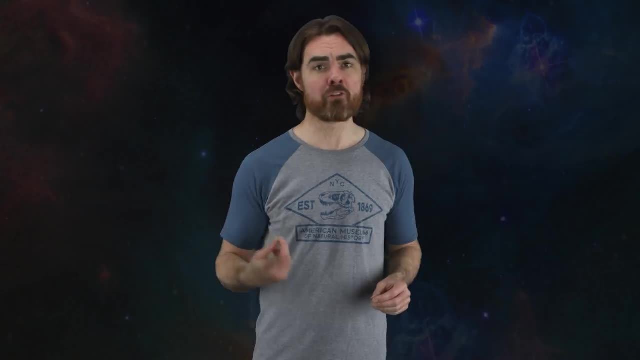 The second quantization approach is the same as the first one, but with a different rules for the fields. 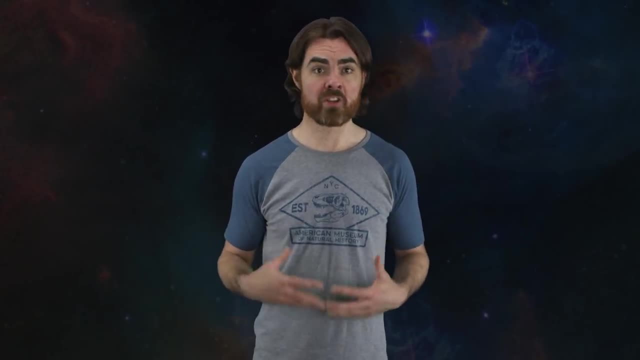 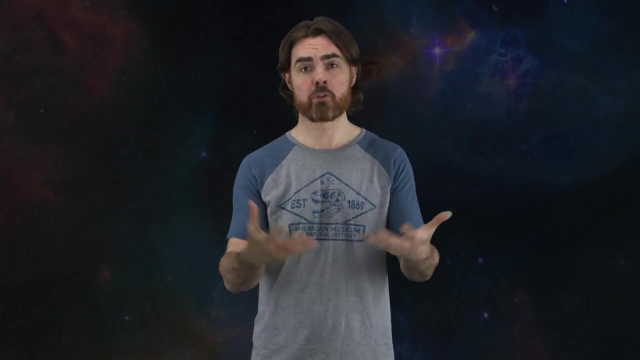 For example, the Pauli exclusion principle tells you that you can only have one fermion, so electron, quark, et cetera, per quantum state, rather than infinite particles in the case of the photon. 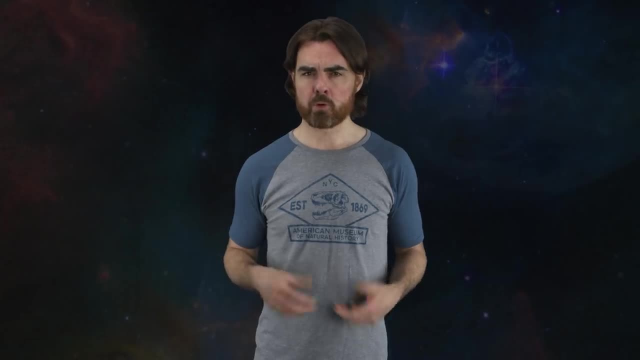 Nonetheless, second quantization works for all elementary particles. That tells us something extremely important. Remember. All particles are also oscillations in fields. 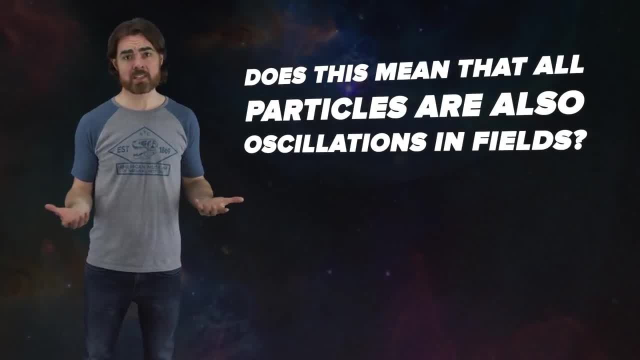 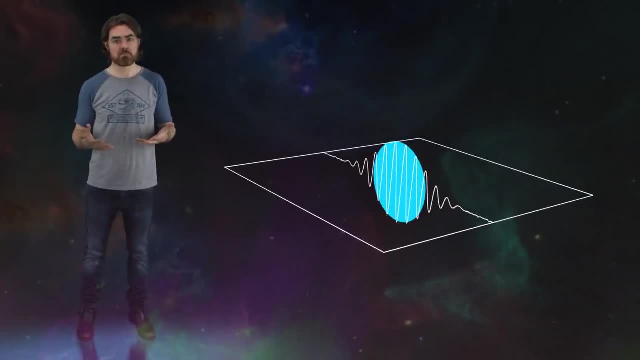 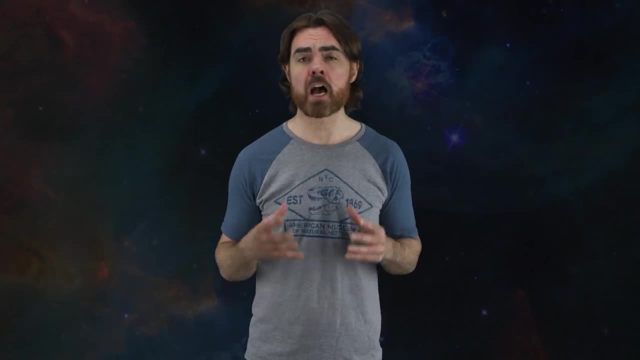 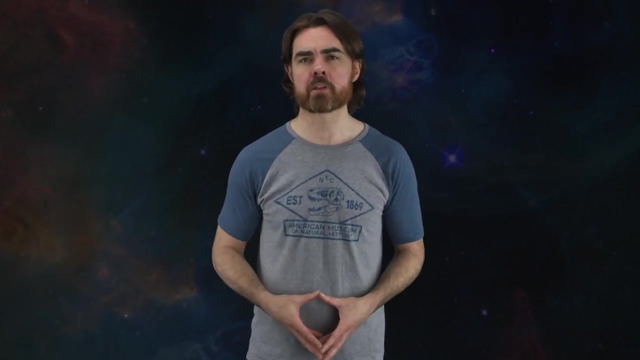 Well, yes, that's exactly what it means. In fact, every base elementary particle has its own field. It is its own field. This is the postulate of quantum field theory. Fields are fundamental. And particles and their antimatter counterparts are just ways in which that field vibrates. There's an electron field, which is a quantum field that vibrates. There's an electron field, whose oscillations 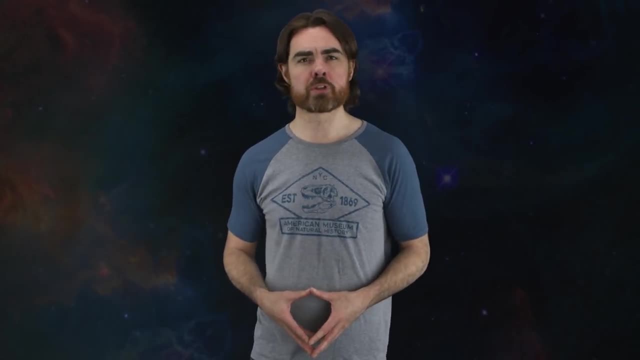 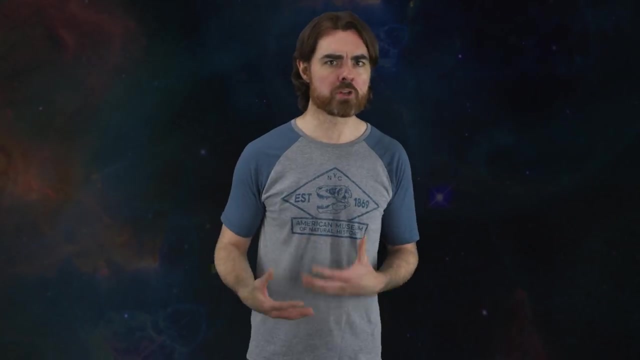 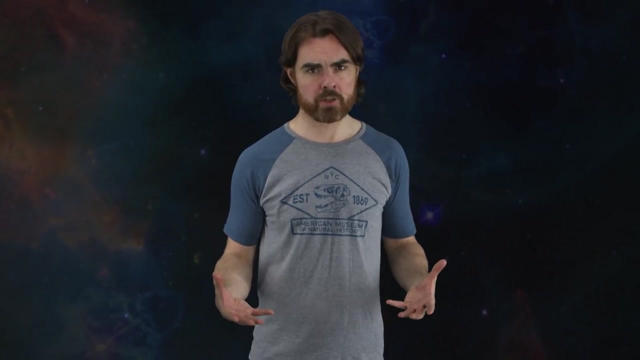 are what we know as the electron and the anti-electron. There are fields for every type of quark, anti-quark pair, for every type of force-carrying particle, so-called bosons, like photons and gluons, and of course, for the famous Higgs boson, which is just an oscillation in the Higgs field. 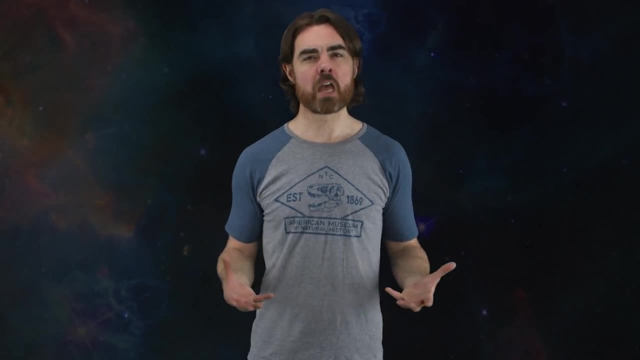 The calculations of QED and of all quantum field theory are about counting the number of ways a quantum phenomenon can occur. 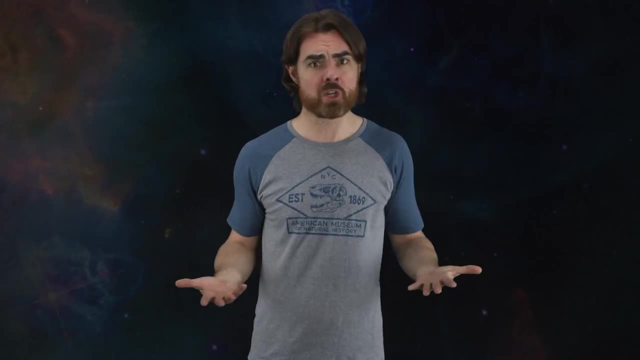 That's a challenge because there are infinite ways in which anything can occur. 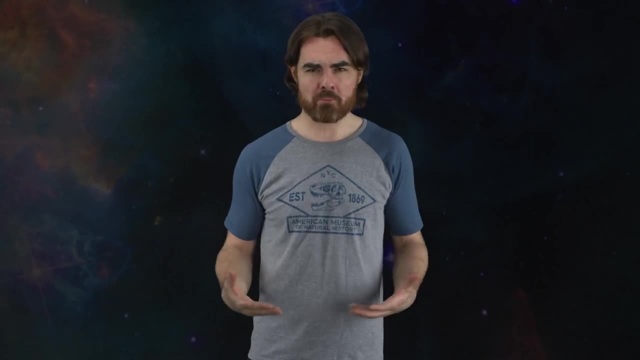 In fact, a huge part of quantum field theory is about taming the infinities that arise in any calculation. 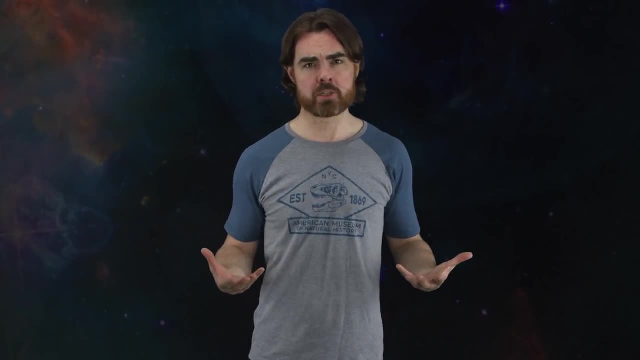 To do that efficiently, we are going to need another genius. We're going to need Richard Feynman. And we're going to need another episode of Space Time. 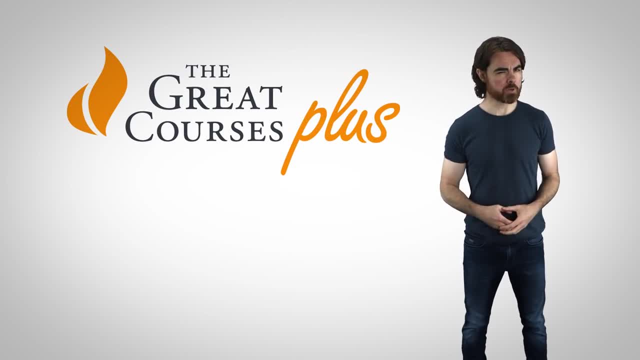 Thanks to The Great Courses Plus for sponsoring this episode. The Great Courses Plus is a production of the Center for Science and Technology at the University of New York. 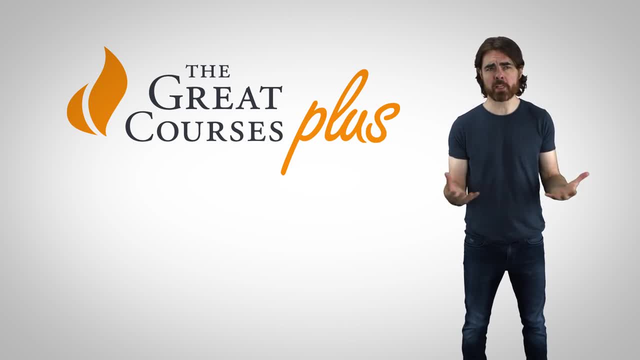 The Great Courses Plus is a digital learning service that allows you to learn about a range of topics from Ivy League professors and other educators from around the world. 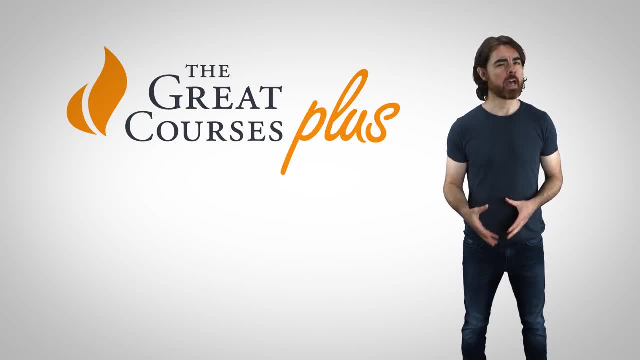 Go to thegreatcoursesplus.com slash spacetime and get access to a library of different video lectures about science, math, history, literature, or even how to cook, play chess, or become a photographer. New subjects, lectures, and professors are added every month. 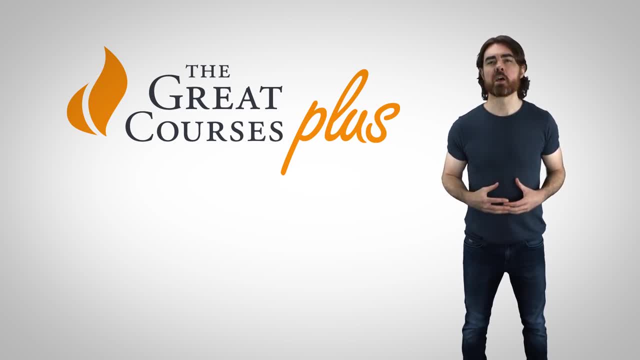 If you want to learn more about the relationship and the conflict between quantum mechanics and relativity, check out the course The Theory of Everything by Professor Don Lincoln from Fermilab. It'll give you some really important background for some of the stuff we talked about today, plus going into some fascinating details that we won't get to. 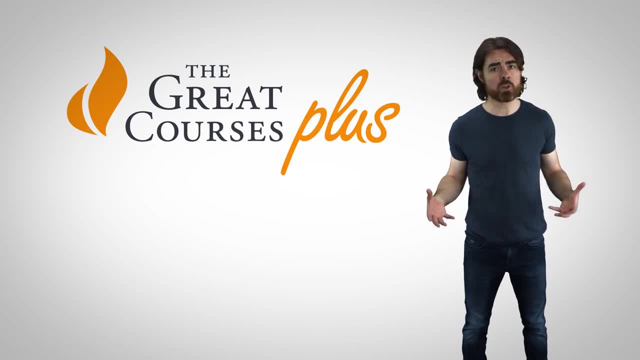 With The Great Courses Plus, you can watch as many different lectures as you want, anytime, anywhere, without tests or exams. 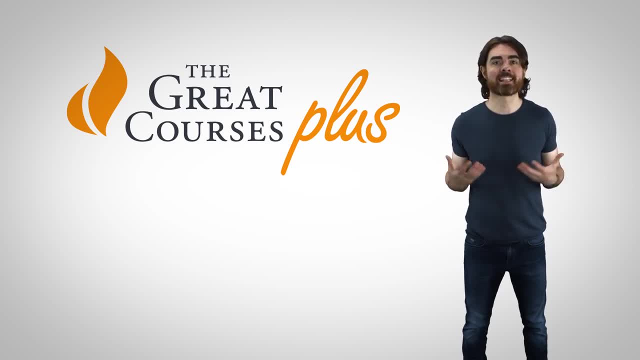 Help support the series and start your free one-month trial by clicking on the link below or going to thegreatcoursesplus.com slash spacetime. 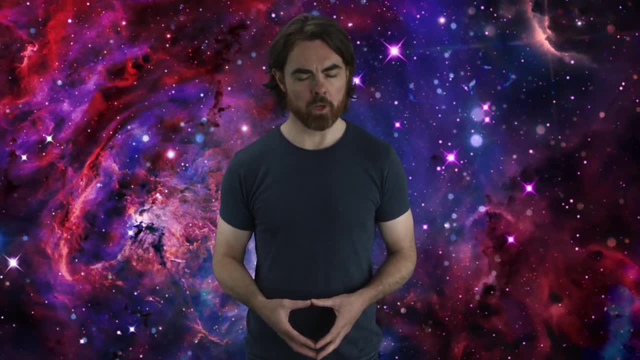 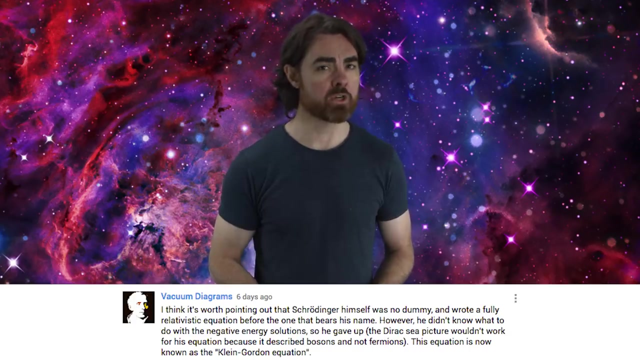 Last week, we began our discussion of quantum field theory by looking at the amazing Dirac equation and how it predicts the existence of antimatter. You guys had a ton to say. Vacuum Diagrams points out that Schrodinger himself did write down a relativistic version of his equation a few years before Dirac came up with the Dirac equation. 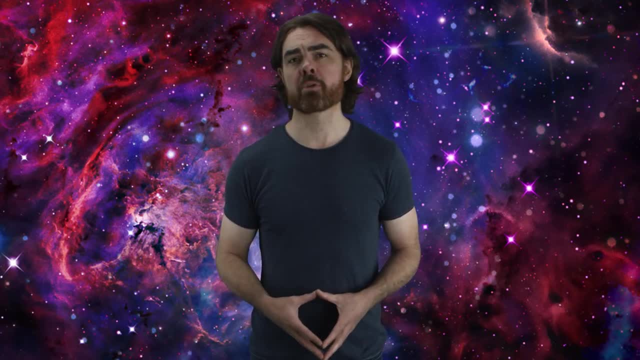 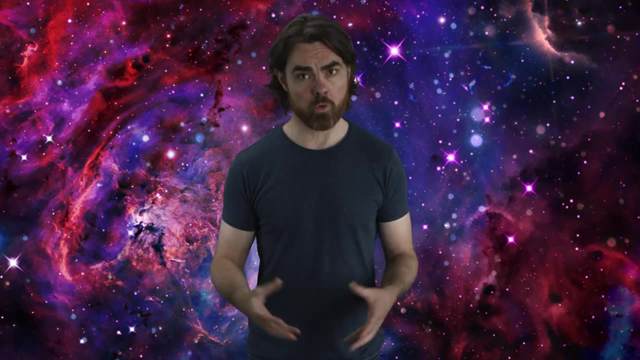 And yeah, that's right. In fact, Schrodinger followed the same approach, starting with Einstein's mass-energy momentum equation. As Mr. Diagrams points out, he said, the resulting Klein-Gordon equation gives negative energy solutions just like the Dirac equation does, but Schrodinger didn't know how to interpret these. It also just didn't work for electrons because it failed to predict the fine structure emission line energies in hydrogen due to not accounting for electron spin. 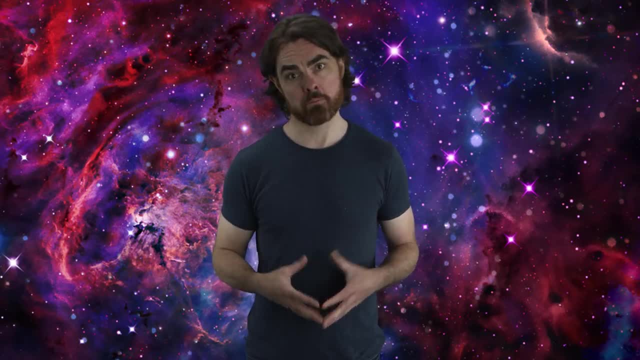 As a result, Schrodinger instead published his non-relativistic Schrodinger equation first. 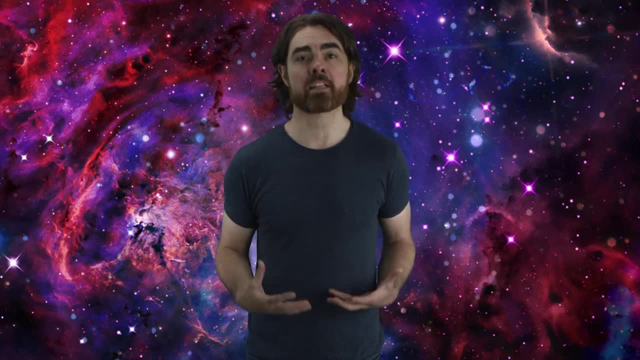 However, the Klein-Gordon equation is actually the exactly right description for particles with no spin. 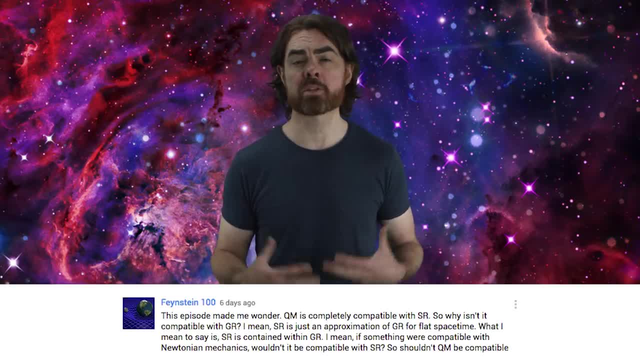 Feinstein100 asks why it was possible to make quantum mechanics compatible with special relativity when we're still struggling to reconcile it with general relativity. 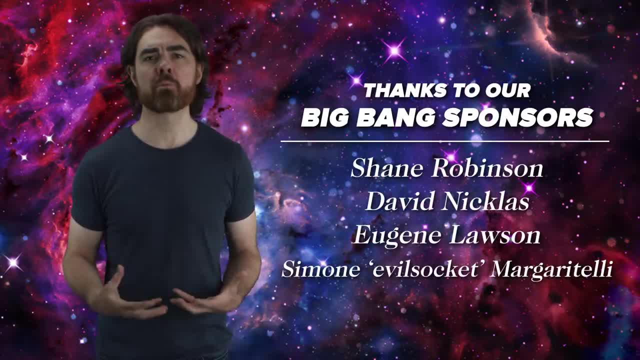 Now, Vacuum Diagrams had a great response that explains the problem of infinities that both special and general relativistic corrections tend to introduce into the theory. 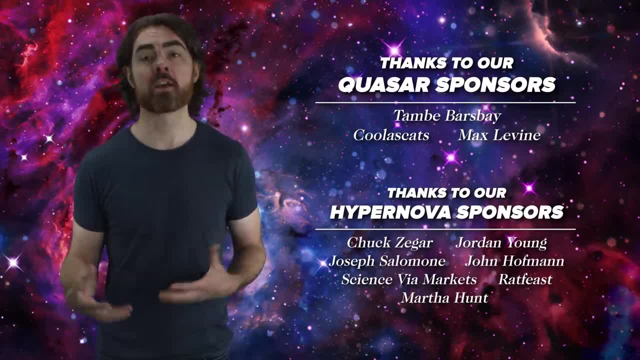 We'll talk more about how the special relativistic infinities were fixed next time using a process that's going to help us in the process called renormalization. 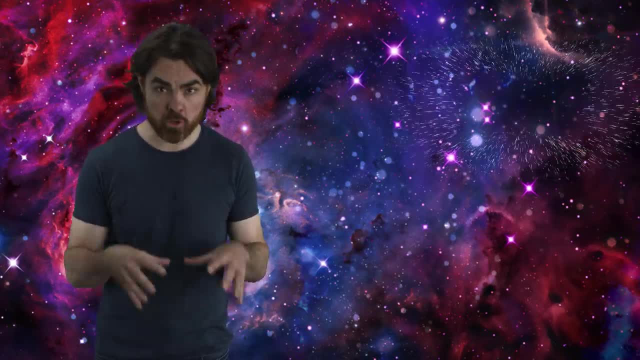 But this trick doesn't work for the infinities you get when you think about curved space on the quantum scale. 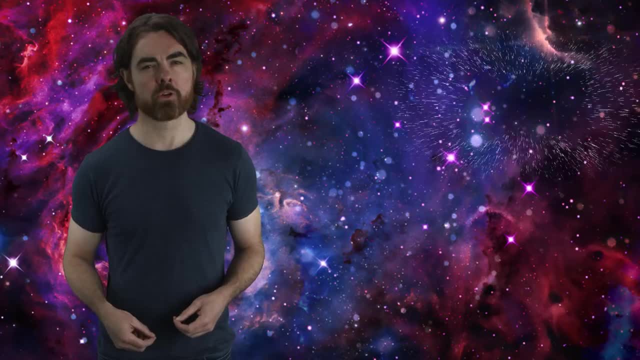 And that's also something we'll get to, but a bit further in the future. 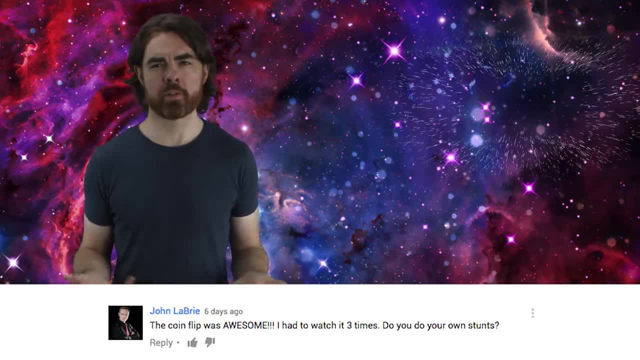 A few of you asked if it took more than one take to catch that coin flip in the last episode. Of course not. It was only one take. 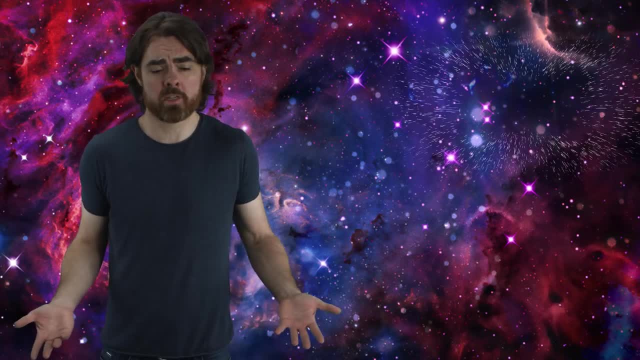 I guess it's possible there are quantum timelines where I missed it on the first attempt, but it wasn't this one. Catch flips. Hey. So, this is a fancy trick, isn't it? And this is a very fun trick. It involves several different functions, even if they don't apply the same thing that you're supposed to do. One, it's the same thing for all the other things that you're supposed to do. And because quantumiałem is a liquid, it's going to be your best trap to capture. So maybe it'll work. Maybe it won't. But instead, you might be able to catch the thing in a lower frequency. You can see, I'm going to catch this one. Trust me, it will. It's a very interesting trick, but I'm not sure why it worked this way. I'm going to give you an example. So if I were to catch a coin making a half-hour curve, 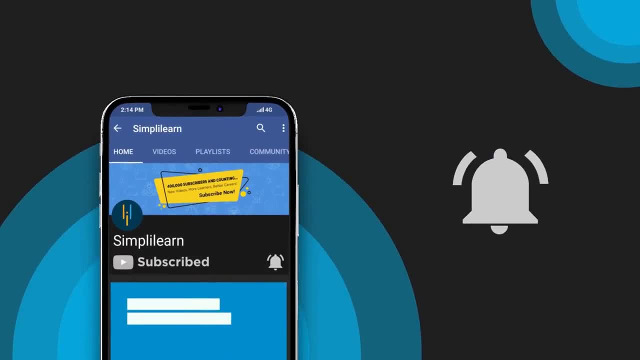 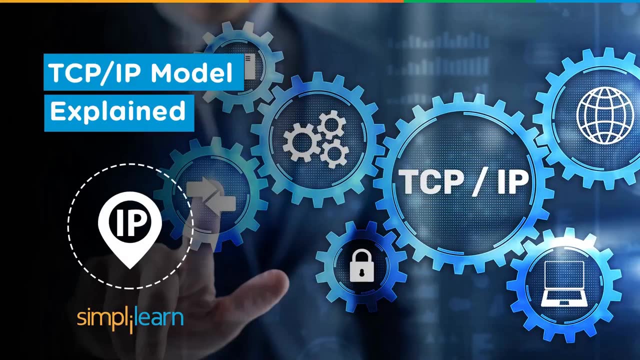 During the transaction of data and information between multiple devices, the task of establishing, maintaining, and the sharing of data is handed over to the network model, which also governs the protocols enacted on the transmitted data. 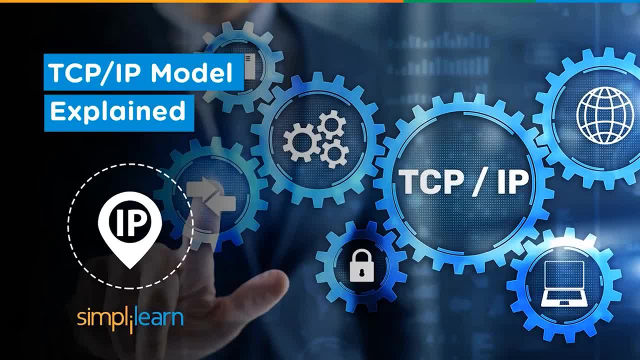 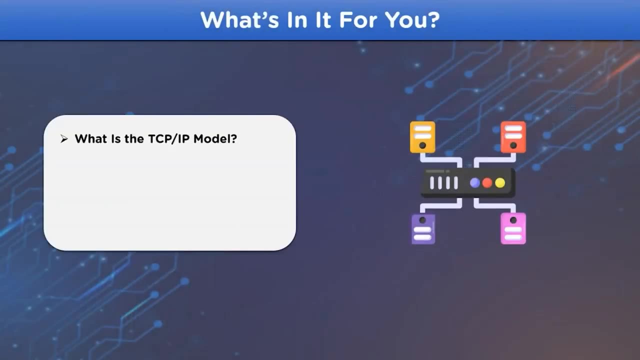 Hi guys and welcome to yet another interesting video on Simply Learn. And before we begin, if you love watching tech videos, subscribe to our channel and hit the bell icon to never miss an update from us. Let's take a look at the agenda for today's session. For today's session, firstly, we'll understand what exactly is the TCP IP model, continuing with the protocols that are applied, the layer structure in the TCP and IP model. 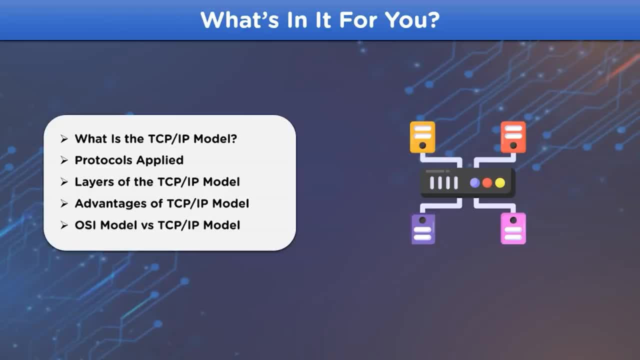 Then we'll see the benefits of using TCP IP model and comparison between OSI model and TCP IP model. Let's begin. Firstly, we'll understand what exactly is the model. The TCP IP model is a method of sharing data and information over the communication channel, where the data has to go through each of the four layer structure of the network model, where it also performs tasks such as remodeling of data, efficient transmission, and error-related issues. Each layer has dedicated protocols that they enact on the transmission.